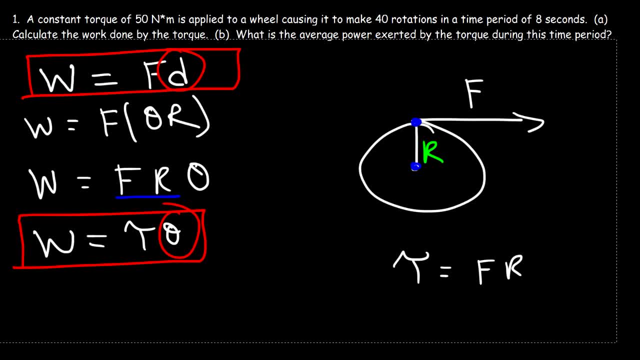 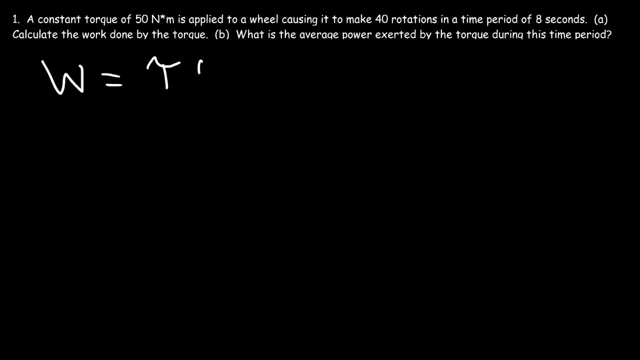 displacement. So now we can finish the rest of this problem. So the work done by the torque is equal to the torque times, the angular displacement. Now we need the angular displacement to be in radians. Right now we have rotations, So one rotation which is equivalent to a revolution, is equal to 2 pi radians. So 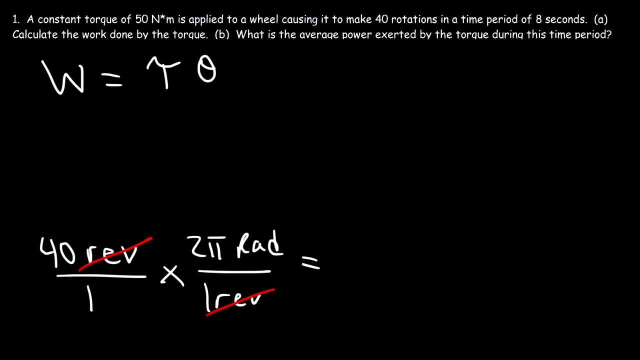 all we got to do is multiply 40 by 2 pi, and so that's 80 pi radians. 80 pi as a decimal is 251.33 radians. So that's the angular displacement in radians. Now we can calculate the work done by the torque. So the torque is 50 newton meters. We're going to multiply it. 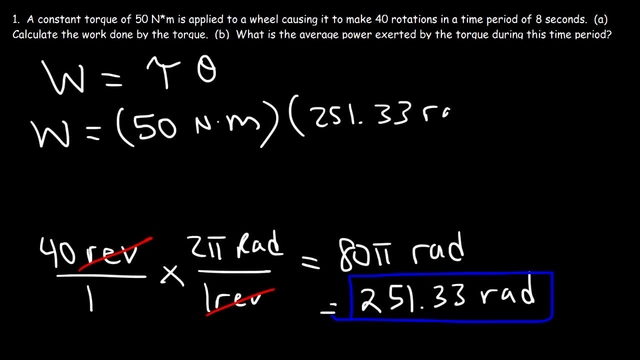 by 251.33 radians, So the work done is 12,500, and I'm going to round it 570 joules. I really have 12,566.5, but I decided to round it a little. So now you know how to calculate the work done by the torque. 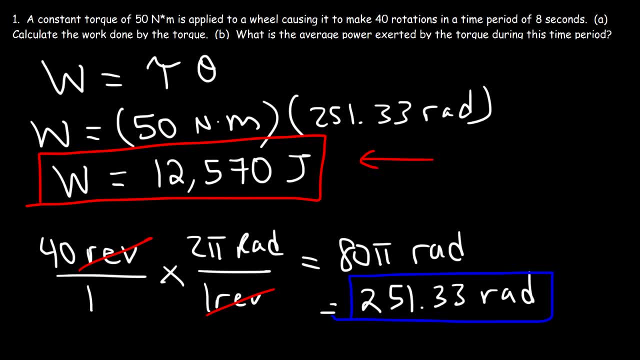 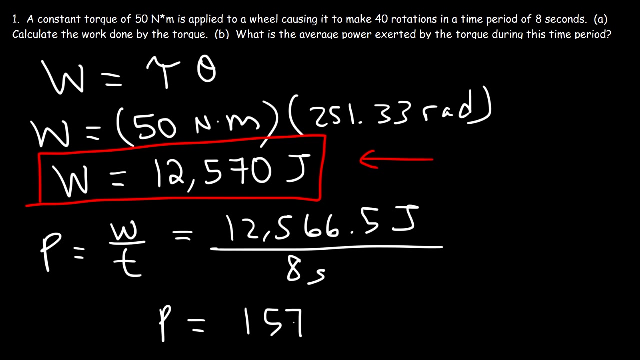 So what is the average power exerted by the torque Power is work divided by time. So work was 12,566 joules. That's the more accurate answer And we need to divide it by the 8 seconds. So the power is 15,000, I mean 1570.8 watts. 1 joule per second is equal to 1 watt. 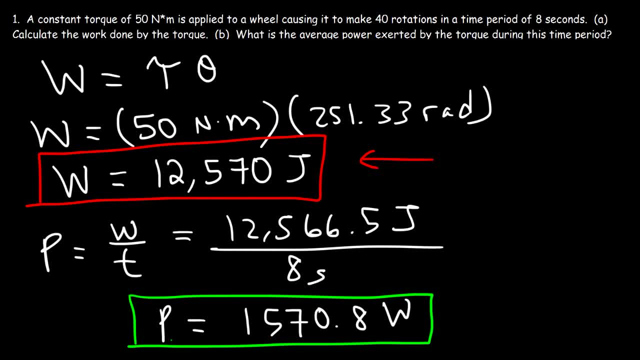 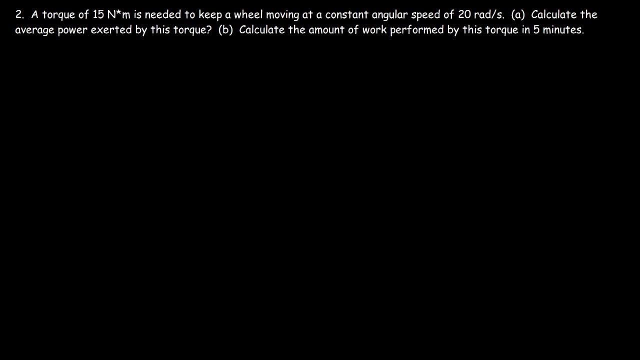 So that's how you can calculate the average power exerted by a torque. It's simply the work done by the torque divided by the time. Number two: A torque of 15 newton meters is needed to keep a wheel moving at a constant angular speed of 20 radians per second. 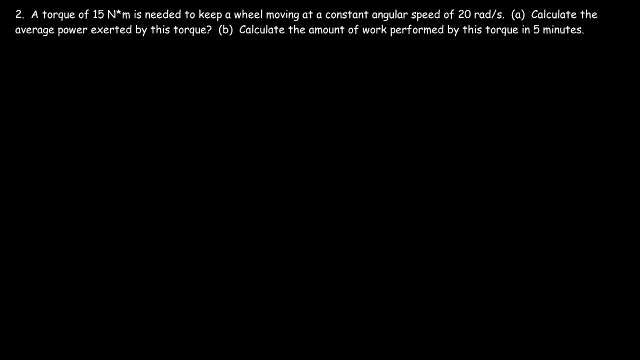 Calculate the average power exerted by this torque and calculate the amount of work performed by this torque in five minutes. So we know that average power is work divided by time And the work done by a force is the torque times the angular displacement, The change in the angular displacement divided by the. 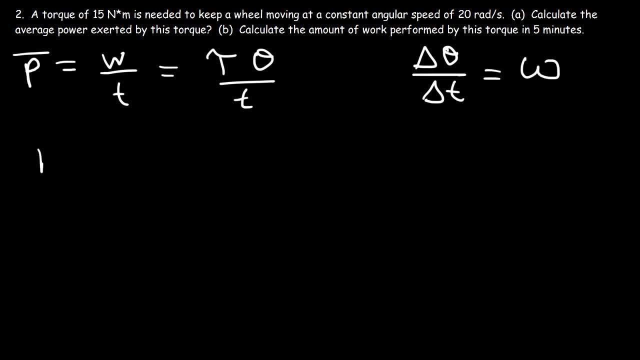 change in time is equal to the angular velocity. So average power is equal to torque times angular velocity. So in this example we have a torque of 15 newton meters and an angular speed of 20 radians per second. So if we multiply these two, this will give us the average power. 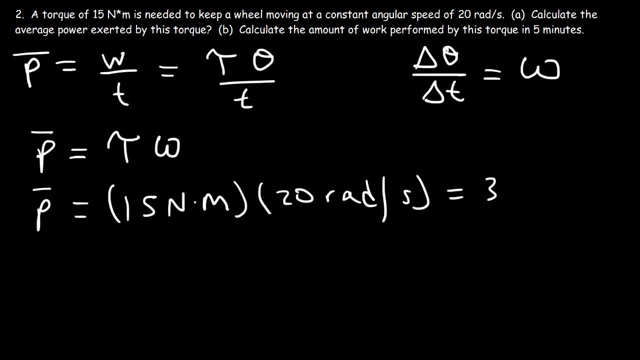 So it's 15 times 20, which means we have an average rotational power of 300 watts, or 300 joules per second. Now part B: Calculate the amount of work performed by this torque in five minutes. So we want to find work. We know that power is work. 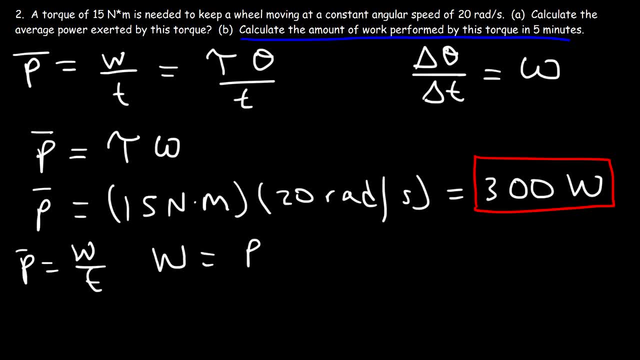 divided by time. So work is power multiplied by time. So let's start with the time in five minutes. Let's convert that to seconds. There's 60 seconds in one minute. So 5 times 60 means that five minutes is equal. 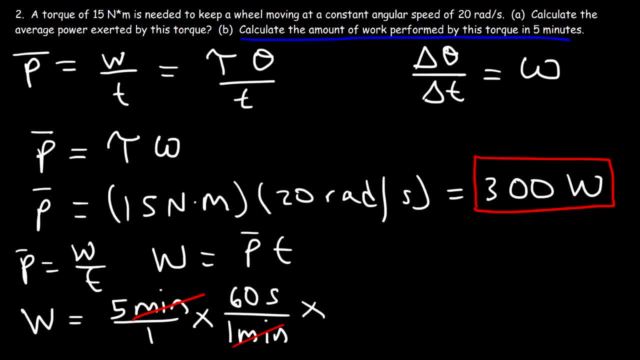 to 300 seconds. Now let's multiply the time in seconds by the power in watts. So 300 watts is basically 300 joules per second, And if we multiply it by 300 seconds, that will give us 90,000 joules. 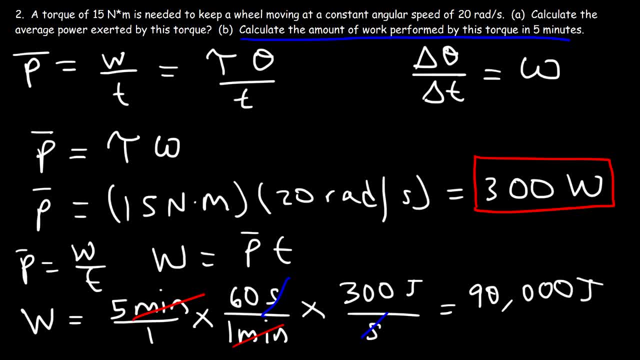 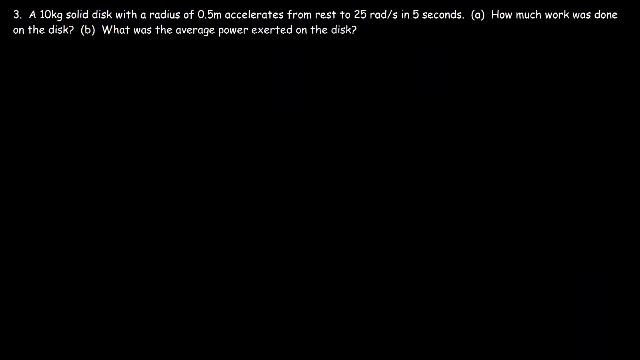 So that's the rotational work done by this torque in five minutes. Number three: A 10 kilogram solid disk with a radius of 0.5 meters accelerates from rest to 25 radians per second in five seconds. How much work was done on the disk? What was the average power exerted on the disk? 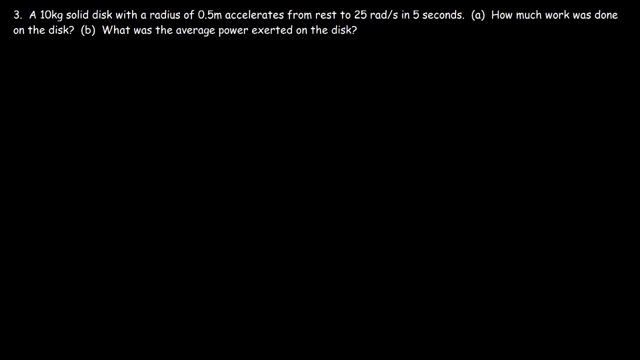 So go ahead and try this problem. Now there's more than one way in which we could calculate the work done by the disk, So this time we're going to use rotational kinetic energy. The work done is going to be the change in the rotational kinetic energy. 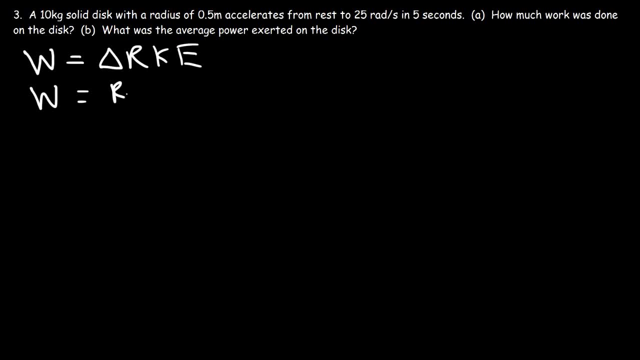 So we're going to use the change in the rotational kinetic energy. So we're going to use the change in the rotational kinetic energy, So it's equal to the final rotational kinetic energy minus the initial rotational kinetic energy. Now the disk is accelerated from rest, so the initial rotational kinetic energy is 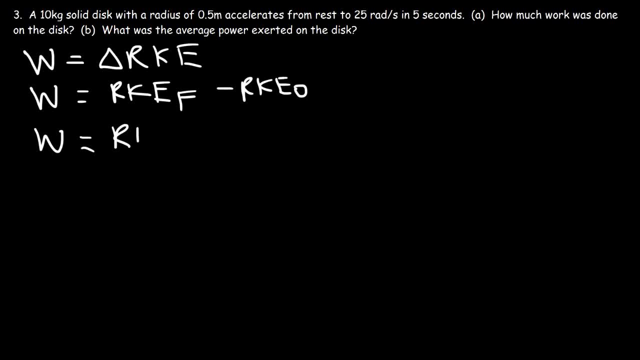 zero. So the work is equal to the final rotational kinetic energy, which is one half inertia times omega, final squared. Now we need to calculate the inertia of the solid disk, So it's one half inertia times omega, final squared. So the mass of the disk is 10 kilograms and the radius is point five. 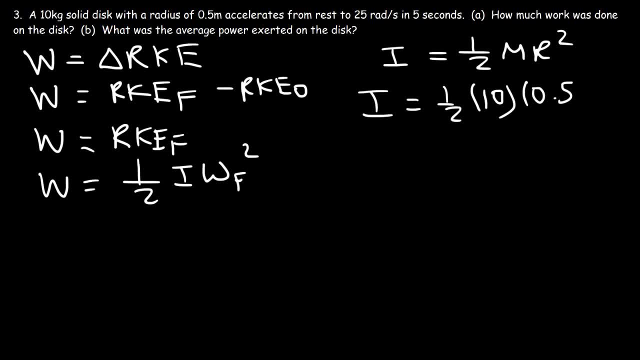 So the mass of the disk is 10 kilograms and the radius is 0.5.. Half of the 10 is five, and five times point five squared is 1.25.. So the inertia is one point 25 kilograms times square meters. 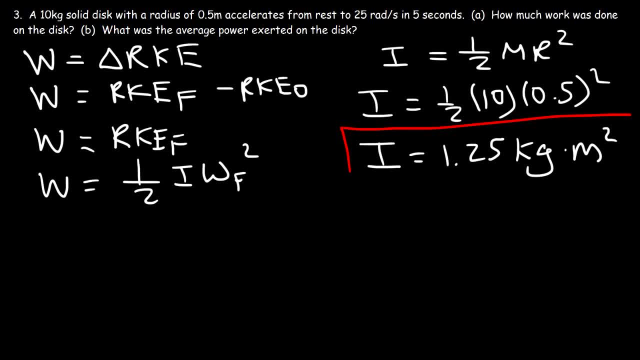 bup 42. So now that we have the inertia and we also have the final angular squared. So now that we have the inertia and we also have the final angular squared, now we can calculate mirror mass, final angular speed, we can calculate the work done on this disk. So it's going to. 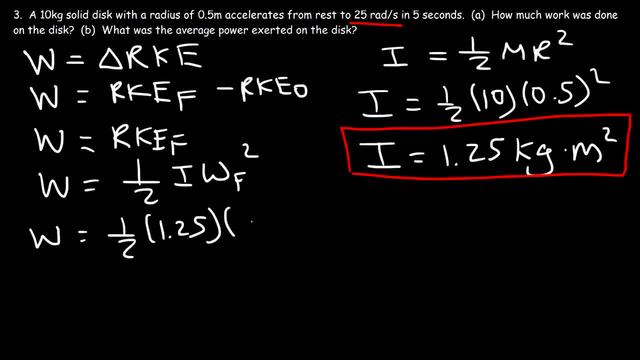 be 1 half times 1.25 multiplied by 25 squared, So the work done is 390.625 joules. So this is the answer to part A. Now part B: What was the average power exerted on a disk? As we know, average power is work over time, So the work is. 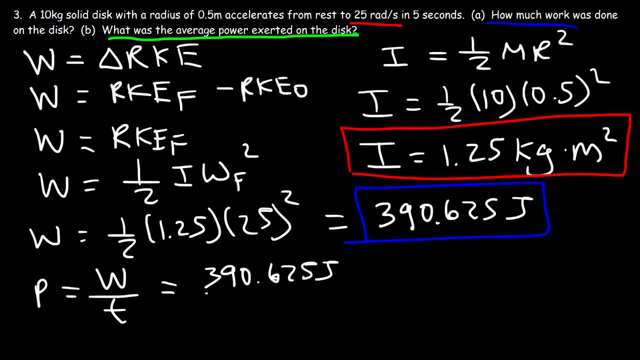 390.625 joules. So the work done on this disk is 390.625 joules. So this is the answer to part A. So the work done on this disk is 390.625 joules divided by a time period of 5 seconds. 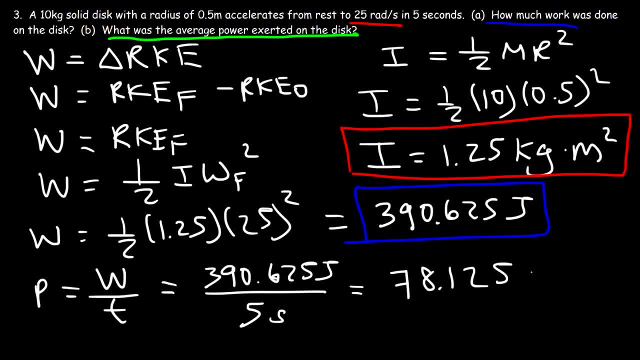 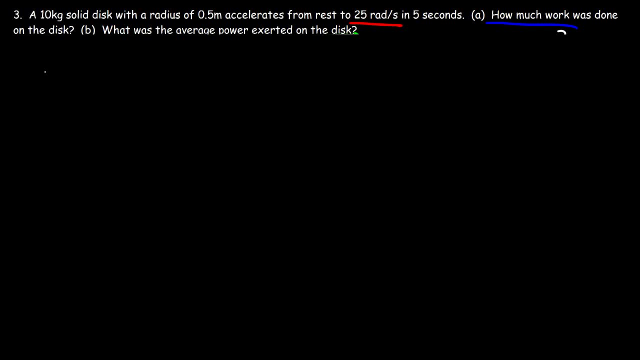 So that's going to be 78.125 watts. Now let's see if we can get the same answer using some other formulas. Now we could also use this formula to calculate the work. It's torque times angular displacement, And torque is inertia times alpha. So we already have the inertia: It's 1.25 kilograms times. 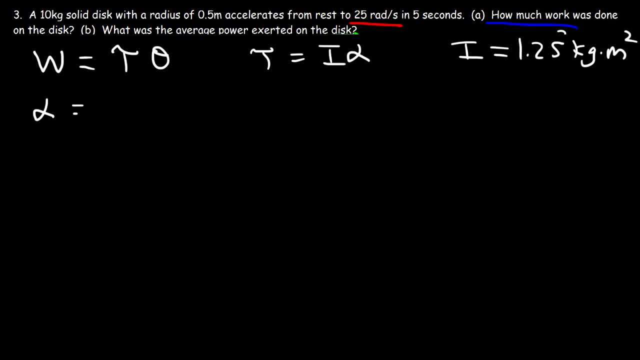 square meters. Let's calculate alpha. The angular acceleration is the change in the angular velocity divided by time. The final angular velocity is 25.. The initial is 0.. And the time is 5.. So it's 25 divided by 5, which is 5 radians per second squared. And so now we can use this. 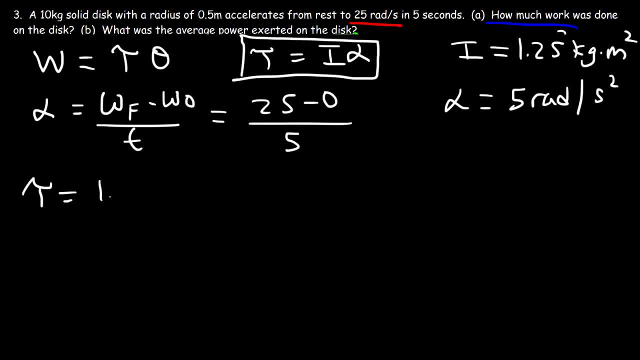 equation to calculate the torque. So the torque is going to be the inertia times alpha, 1.25 times 5.. And so that's going to give us a torque of 6.25 Newtons times meters. So now the next thing we need to do is to calculate the angular displacement. 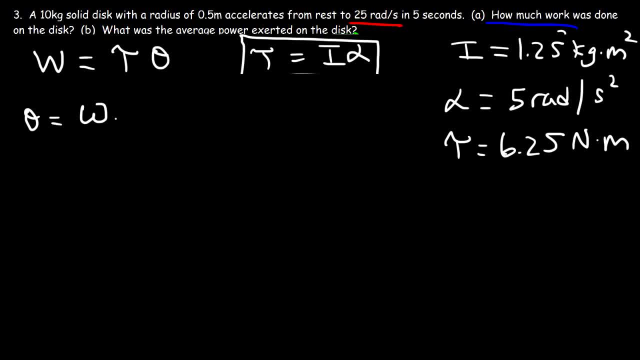 So we could use this formula to do so. It's equal to Omega initial times T plus one-half alpha T squared. Now, the initial angular speed is 0,, alpha is 5, and t is 5.. So it's 5 times 5 squared, which is 125, and then divided by 2.. 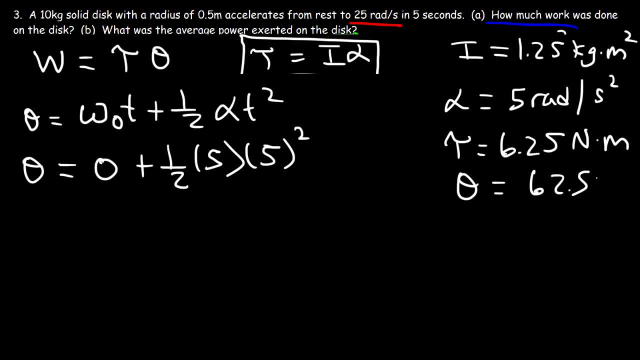 So the angular displacement is 62.5 radians. So now we can calculate the work done by this torque. So it's going to be the torque which is 6.25, times the angular displacement of 62.5.. And so the work done is going to be 390.625 joules, which is an answer that we got earlier. 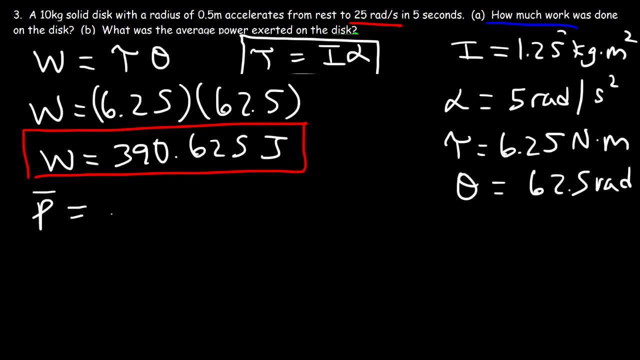 Now to calculate the power. average power is going to be equal to the torque times the average angular speed, And the average angular speed is basically the initial plus the final angular speed divided by 2, which is the same as multiplying it by 1 half.